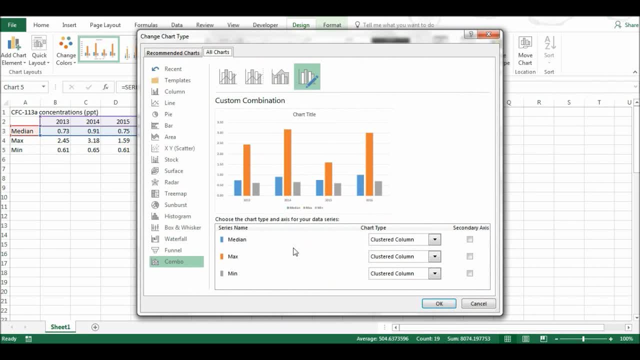 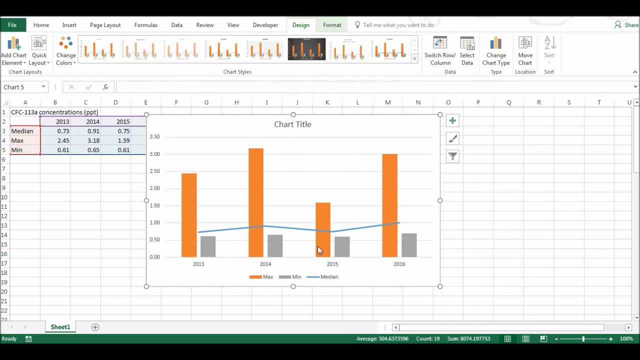 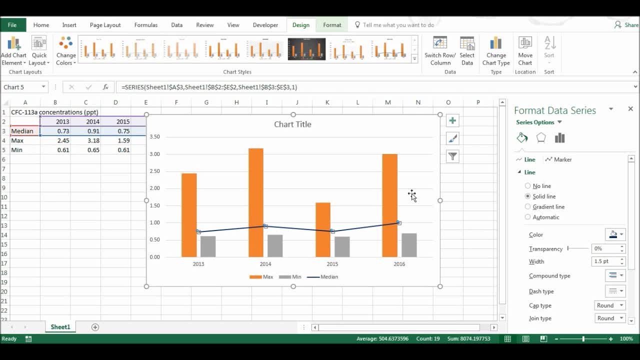 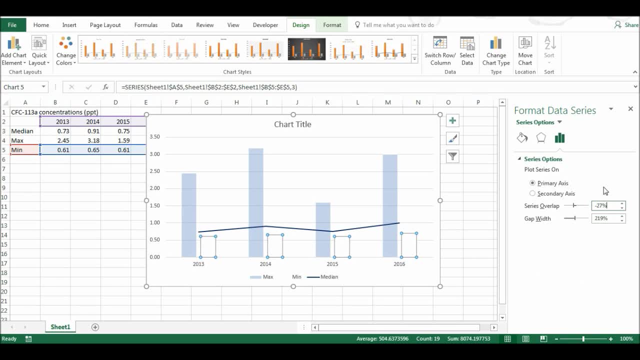 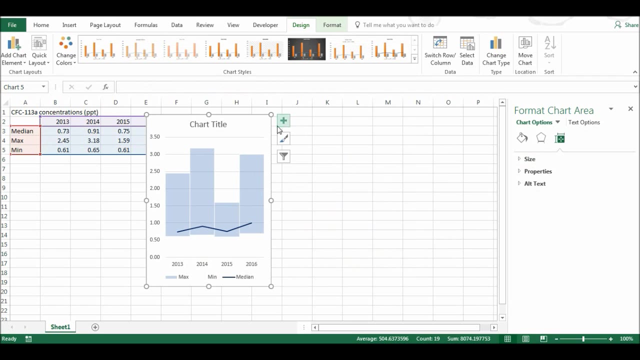 Then I'm going to go up here. I'm going to change these series overlap to 100%, Then I'm going to change the gap width to 0%. Now I'm going to make the chart a little bit skinnier So it looks a bit more in proportion, and 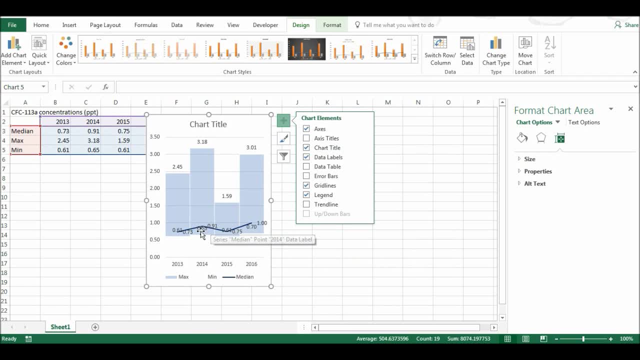 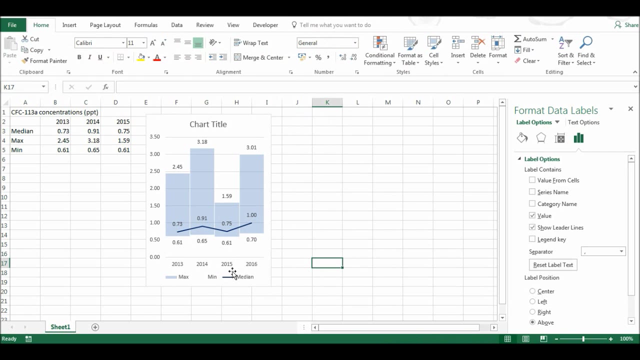 I'm going to add data labels. Now I'm going to move the data labels, so I'm going to get the minimum values to be inside end and Then the median values to be above the line. Now I'm just going to delete some of the features that I don't want. So I don't want the legend. 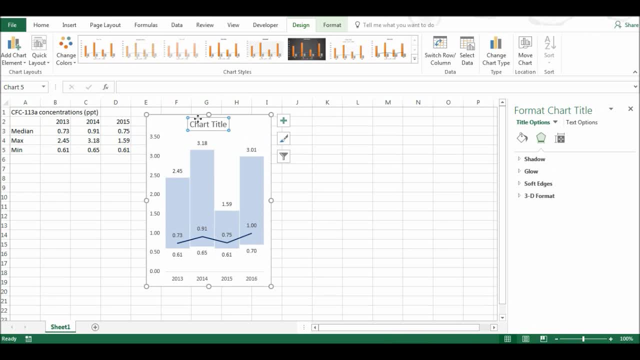 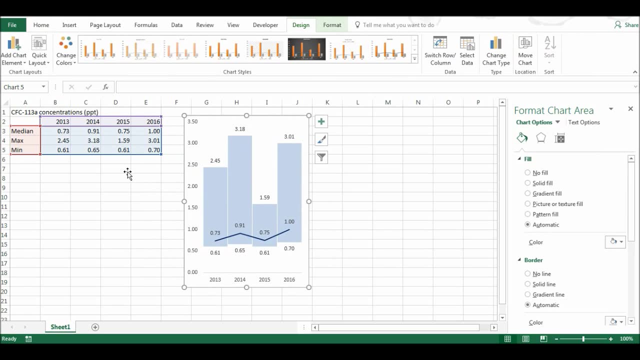 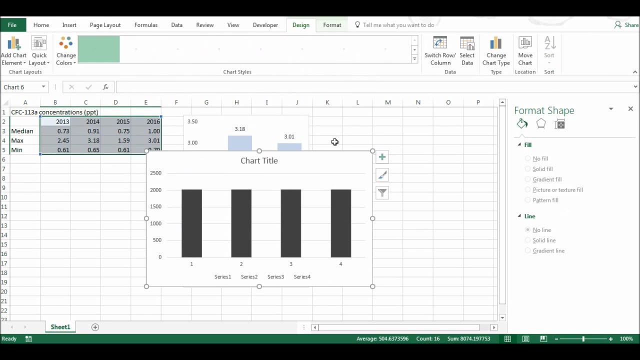 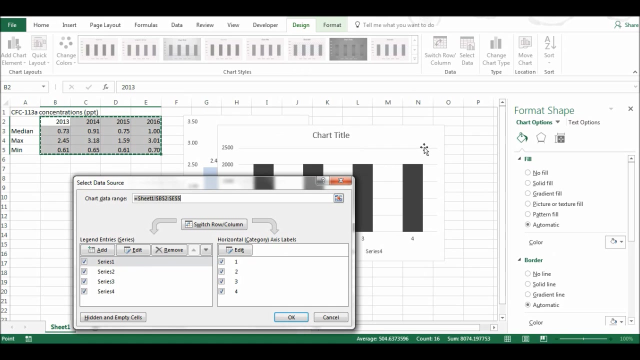 Or the grid lines Or the title. Okay, and there's the first graph. Now I'm going to make the second graph. I'm going to highlight all of this data and go to insert and this time make a stock column graph. Now I'm going to right-click on this and select data and I'm going to remove series one. 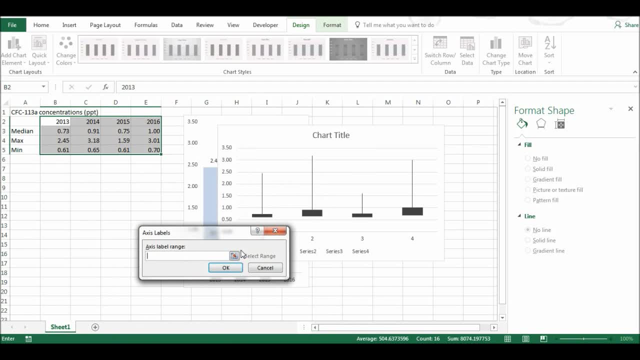 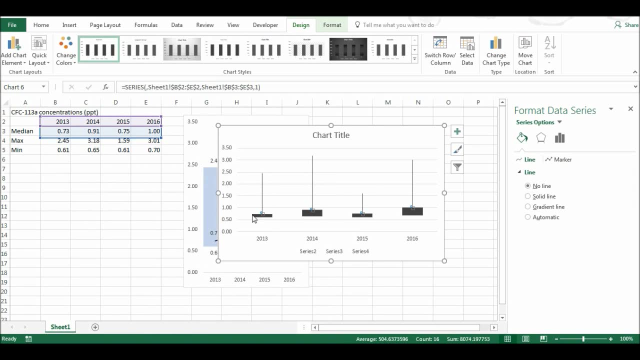 Then I'm going to edit the horizontal horizontal axes to be the years, Then I'm going to select ok and ok again. Now I am going to delete these boxes And I'm going to go up here and I'm going to select a series two and I'm going to make this into a solid line.